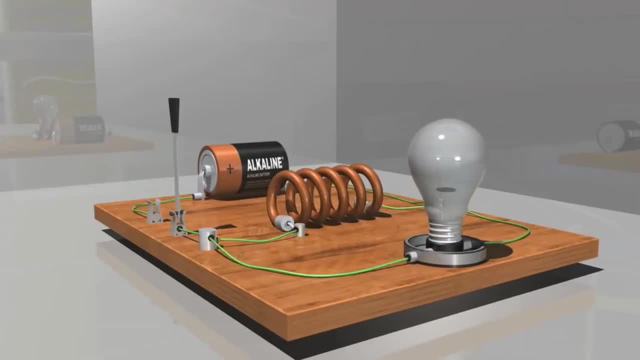 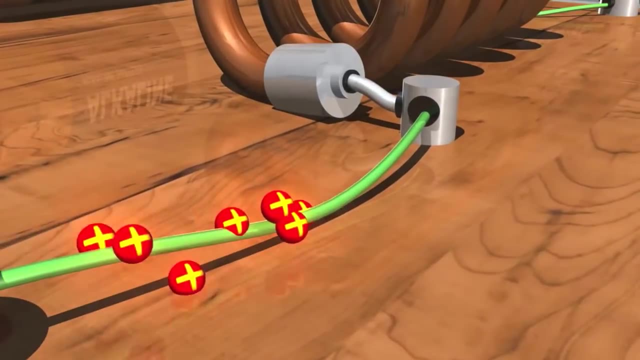 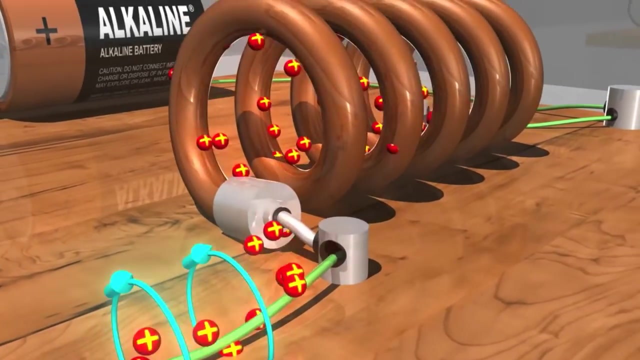 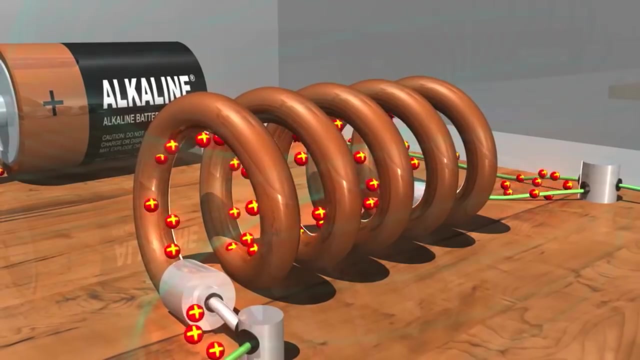 illustrating how back EMF works. When we power this circuit, the electrons in the current create a magnetic field around the wire as they move through it, as shown by these blue arrows. If the wire is formed into a coil like this inductor, the magnetic field lines converge in the center. They gradually 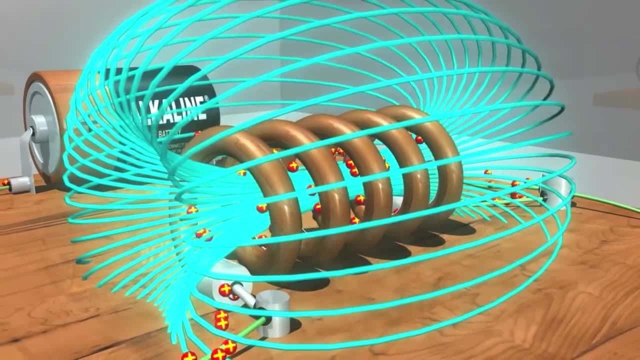 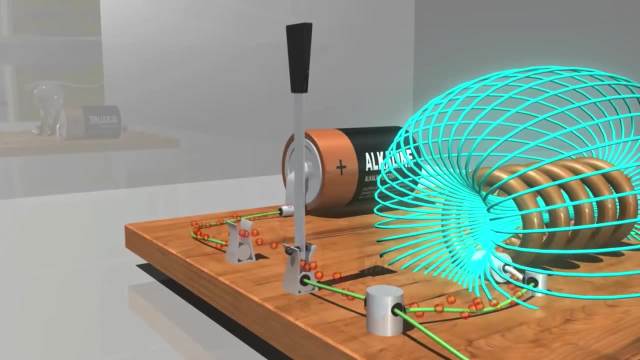 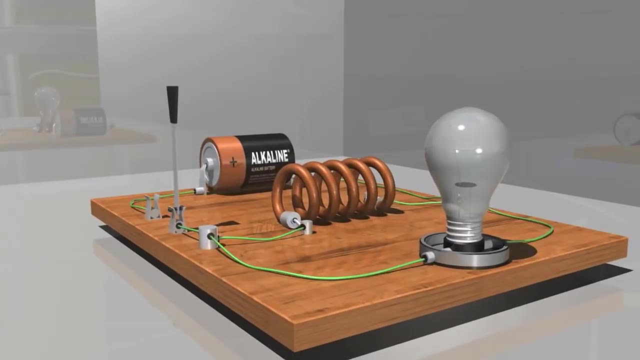 build up to a maximum magnetic field that is much stronger than the one around the straight length of the wire. again, but this time we'll pay closer attention to what's happening in the wire conductor. In this parallel circuit, the current can travel either through the inductor or through. 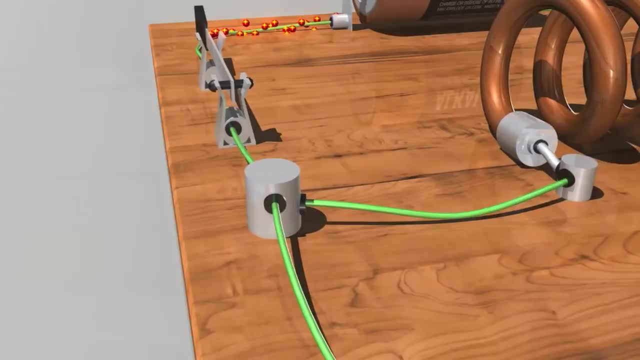 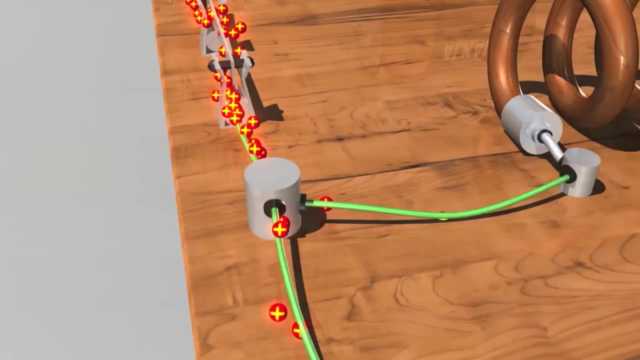 the light bulb. When the current reaches this junction, it splits and flows to both the inductor and to the light bulb. At first, the current flows much more strongly towards the light bulb. This happens because as the magnetic field in the inductor grows, it induces its own. 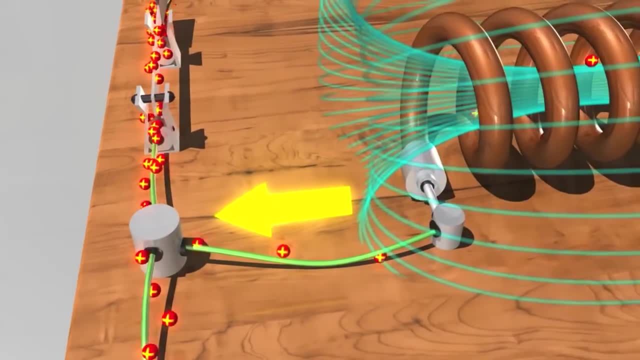 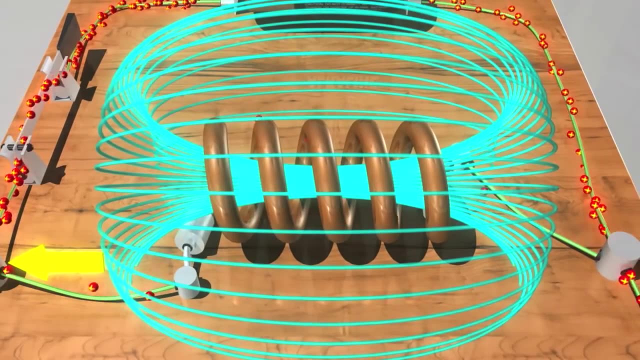 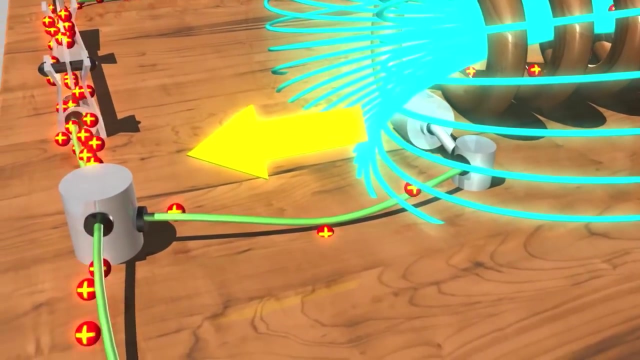 voltage. through Faraday's law This is called electromagnetic induction. So the inductor here is creating a back EMF, represented by this yellow arrow. Back EMF always opposes the change that created it. So in this instance the back EMF is opposing the change. 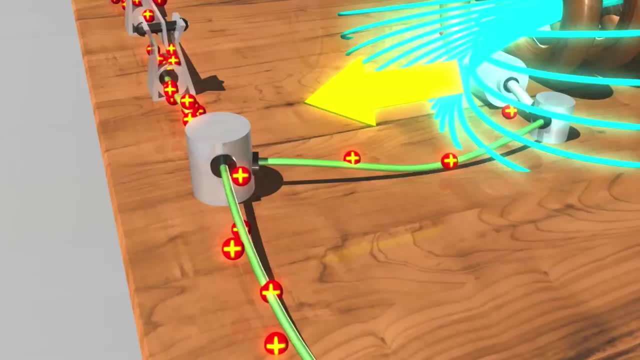 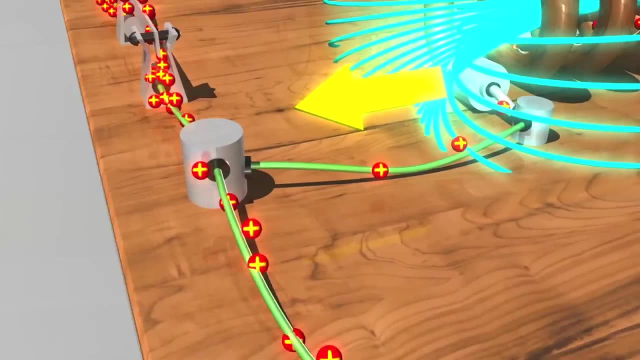 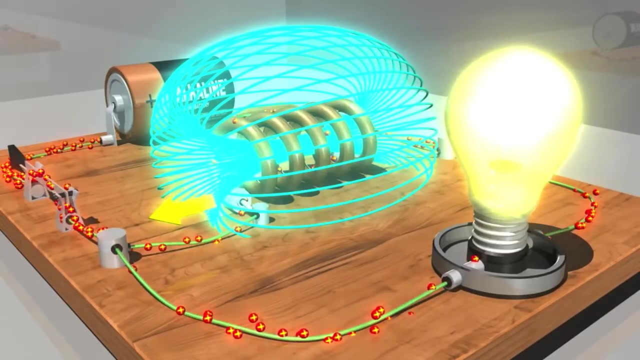 created by turning on the circuit. It opposes the current. The result, as you can see, is that the back EMF effectively diverts the current away from the inductor and toward the light bulb. This causes the bulb to light up, but only briefly. 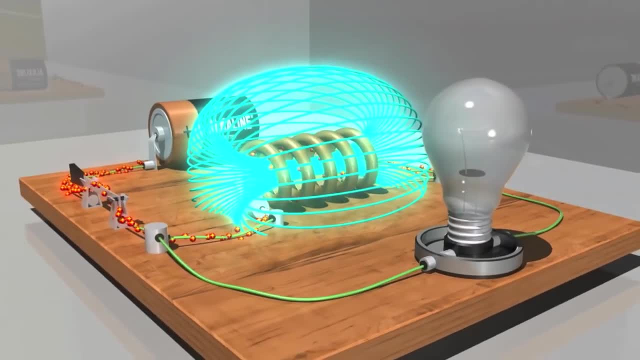 Once the magnetic field around the inductor reaches its maximum field, the back EMF fades and the current now favors the back EMF. The current now composes the back EMF, So the back emf is the back of the inductor and toward the light bulb. 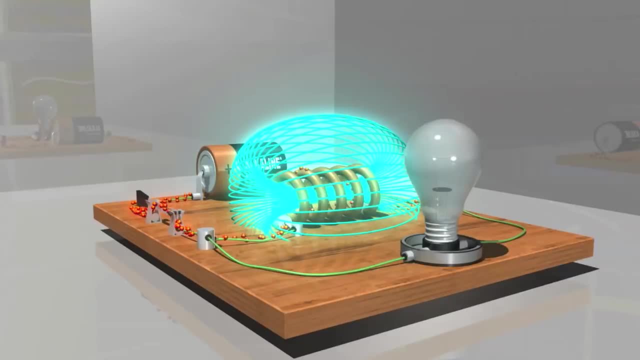 As you see, the back emf turns into two conventional curves. here The back emf is in direct contact with the current. The front emf is in direct contact with the current path through the inductor because the bulb creates some resistance to the current. the same phenomenon.